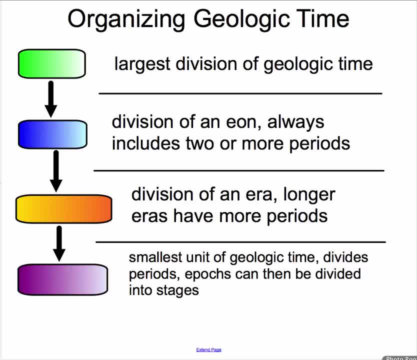 Hi everybody out there, Mr Gilbert and Mr Kimpton. here We're going to do a little bit about geologic time for you today, and we're going to start with how geologic time is organized, and Mr Kimpton is going to kick us off. All right, there's a number of ways to organize geologic. 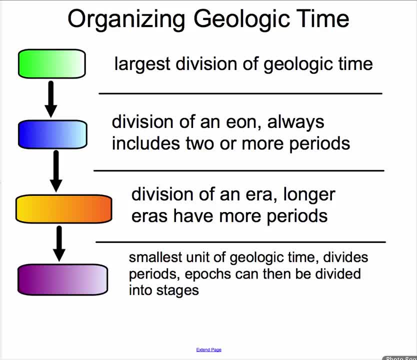 time, and the most common way is through using four different sections or organizing it as if were a book, which Mr Gilbert will talk about. The first way is you start with the largest division of geologic time, that's called an eon. So if geologic time of earth were a book, this 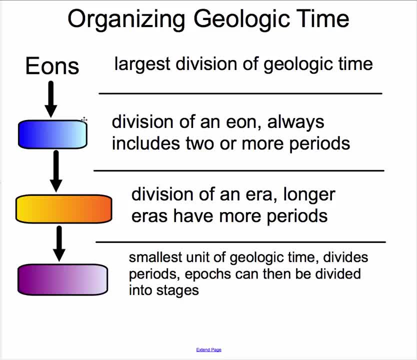 would be like the chapters, dividing big segments of time- eons- And then we take those eons and we break them up into what is used probably the most- and we'll talk about the most, which are eras. And if the earth's time were a book, we would take the chapters. 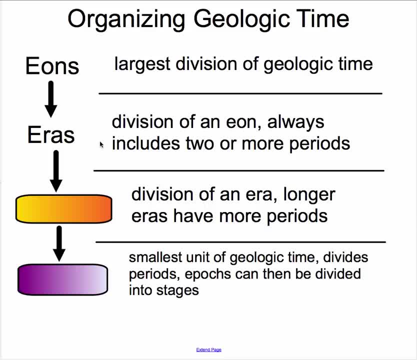 the eons and the chapters and divide them into eras, paragraphs, So paragraphs getting smaller. Then we take those eras and those eras each have- it depends on the era- a different number of periods embedded within them. And if it was a book, these would be sentences, The 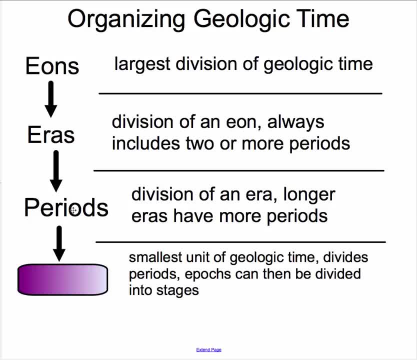 periods would be like a sentence inside of a paragraph, an era inside of a chapter, an eon, And then if you were to really get specific and if you take geology in college, they'll take those periods and break them into epochs. 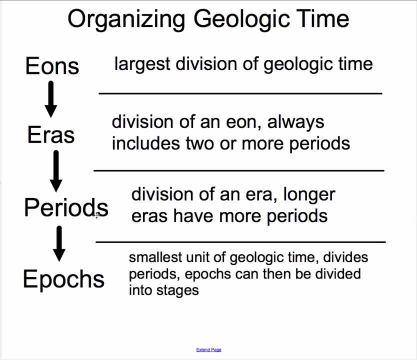 Some people say epochs, but you can decide how you want to say it. They're not used that often. unless you get really specific, It will be real small, like a word within a word, within a sentence, within a paragraph, within a chapter. So geologic time is a lot like reading books. Imagine that. So let's talk. 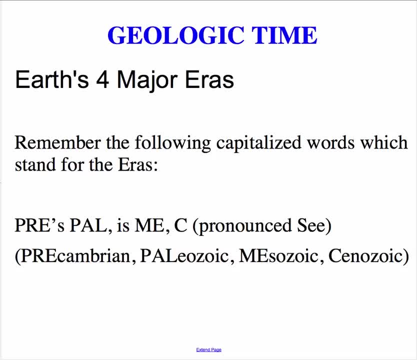 about some of them, more about the earth's four major eras, and technically we're giving you a little baloney right now because there's only three eras, but we're going to lump in an eon as an era. so the way to remember them- you don't know them yet, but just remember them- is by the little moniker pre's. 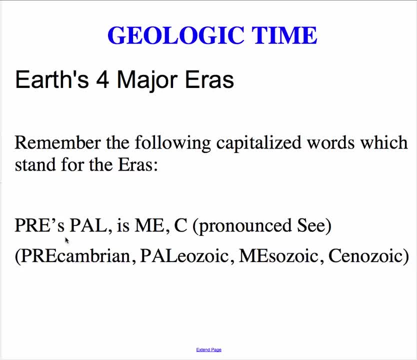 pal is me c, and that's right here on the board. we'll highlight it for you. pre's pal is me c, and that would be the pre-cambrian, the oldest, the paleozoic, the mesozoic and the cenozoic. and these would be the orders from the beginning of, or the eras from the beginning of, history. 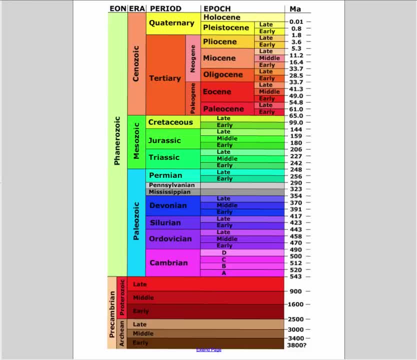 right up until the present and, of course, you can see all this put together. you can go online and find a bunch of resources to show you different ways of dividing things into the different eras and periods, epics, etc, etc. but we're going to hit some highlights for you. 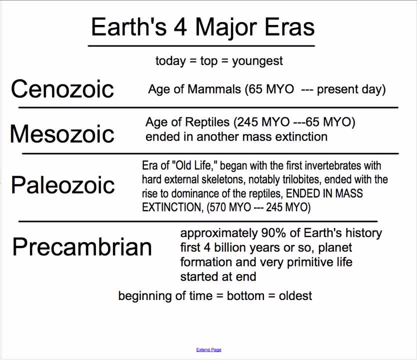 all right. so the way this is set up is using the law of superposition. pre-cambrian is down on the bottom, so we're actually going to talk from the bottom of the page up to the top, because that's how the rocks get stacked up, unless you mess them up. so up at the top you'll see it says: today equals top. 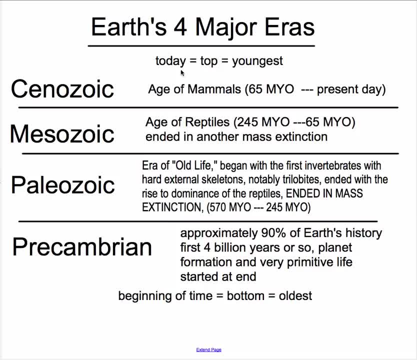 equals youngest. whether we've taught you that part yet or not, here we go. so the pre-cambrian, which means before cambrian, that's approximately 90 percent of earth's history. the first four billion years or so, you and that's uh, primarily the planet formation and very primitive life was starting towards the very 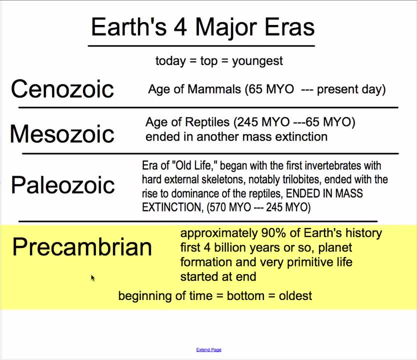 end of that, right before it was called the cambrian explosion. i'll let mr gilbert talk about that. so about 570 million years ago we find a lot of fossilized life, explosion at the beginning of the paleozoic. and i mean life is going nuts. it's growing all over the place, many single-celled. 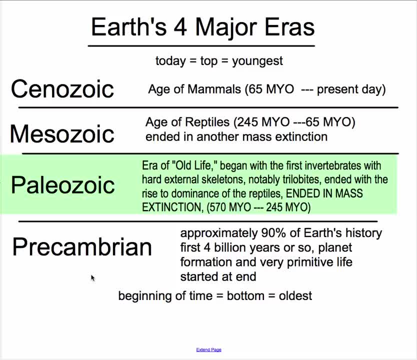 organisms are cruising around, etc. and it's called old life. there's invertebrates, there's hard skeletons like clamshells, trilobites, things that we're going to find, fossil honey, which i'm not going to tell you about, and um, as it keeps. 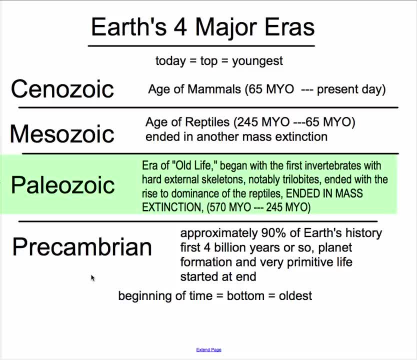 going on. you know life is starting to get crazy and you know life cruises into land and we get some amphibians and plants and crazy things and then, wham, at the end of the paleozoic we get a big extinction, um, probably the biggest one, well, the biggest one we know of on on record, and, uh, that. 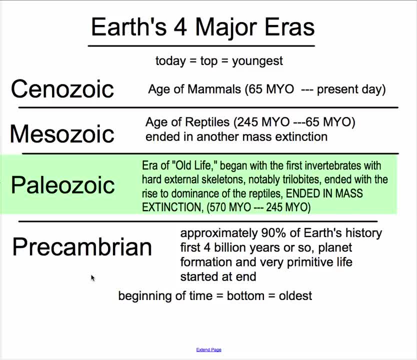 kind of gets rid of a lot of life, and we're going to talk a little bit more about that in just a minute, but i'm going to start with the paleozoic. so you know, the paleozoic is a species of life, about 90. 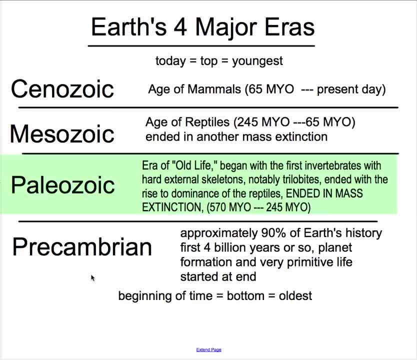 percent of all life ends in the fossil record and it begins the mesozoic era. and that is kind of like freedom for a lot of species that were living under the panic and tyranny of of other species. and mr kimpton's going to get us into the mesozoic. uh, the mesozoic meso means middle and uh, it like 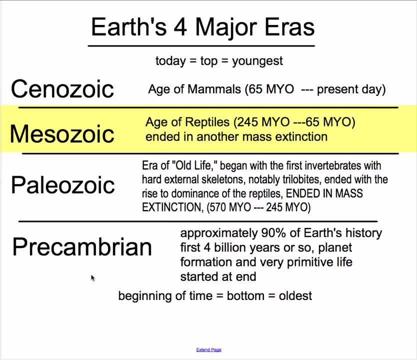 the paleozoic ended in a mass extinction, so you could think of the mesozoic as the middle of two different. certainly, but it is not really an res造 Надanalim, it is it lit, which you are trying to embrace. you're trying to start looking at some very interesting. 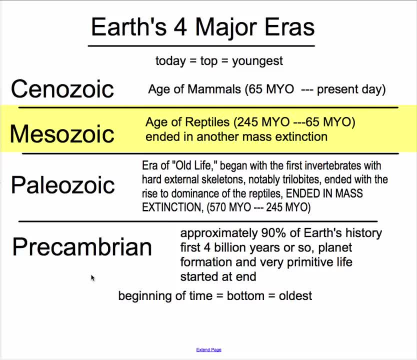 Whoa, have you seen it? but將 we say? but that, that, that this period, whererang, that is the um, when gravities are of your own and when life lightnings hit, uh, you know if it was it, if it was really a time before cleaning up. 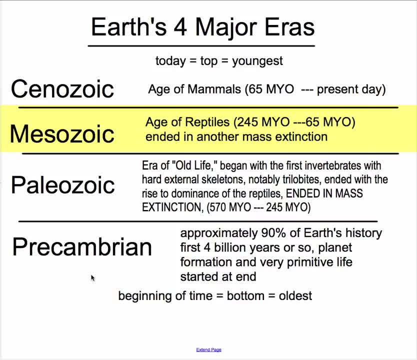 each or multiple soldiers or whatever that might seem like that, then at that point you might have a special nessa in your relation, as much as it used to be. we'd be carrying an old old the end, when the leading theory right now is that a large asteroid impacted. 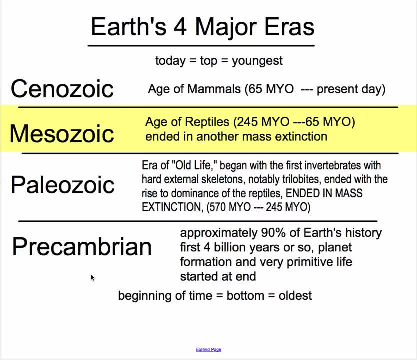 Earth and pretty much changed the climate significantly, so much that too many of them could not adapt in time to survive. I'll let Mr Gilbert talk about the Cenozoic And with a lot of the reptiles and big carnivores out of the 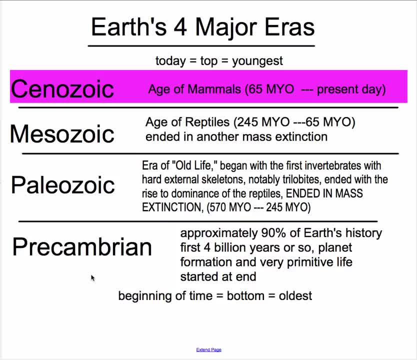 way at the end of the Mesozoic, kind of a lot of these animals and creatures that were smaller could maybe live underground or make their own nests- took over and therefore the age of mammals really started cruising around And some people even throw insects into that And that's the Cenozoic. It's the last 65. 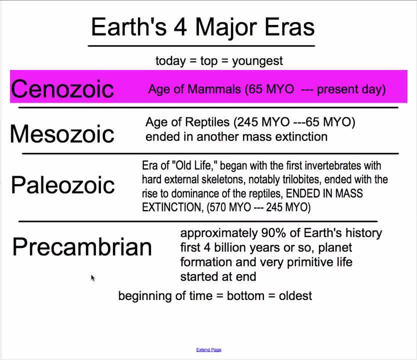 million years of where the Earth went from: a relatively, compared to today, more hot environment down to today it's more cooler environment, including the ice ages that we've had very recently, And the Cenozoic is just a great time. You and 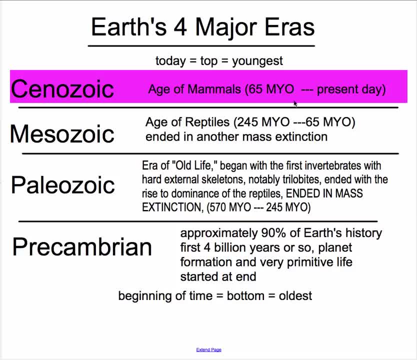 I live here. We live in the Cenozoic today. By the way, if you didn't know, MYO stands for millions years ago, So the Cenozoic started 65 million years ago and is still going on today, And that's it. 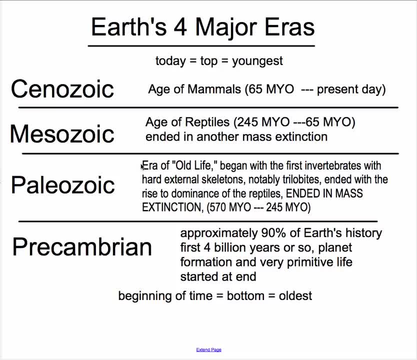 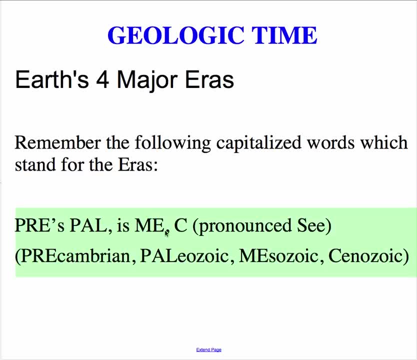 We hope you enjoyed this event. Yes, it's been great. Pre's pal is me C, And that's right here on the board. We'll highlight it for you. Pre's pal is me C, And that would be the Precambrian, the oldest, the Paleozoic, the Mesozoic and the Cenozoic.